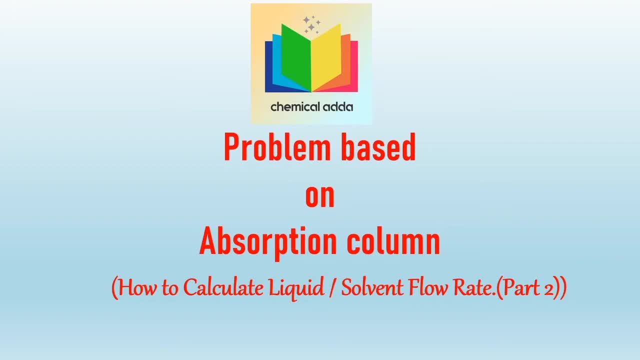 solvent. If you know the answer to any question, Please comment in the comment box And If you like my video, Please like, comment, share And subscribe to my YouTube channel, which is chemical idda. So let's see the first question. 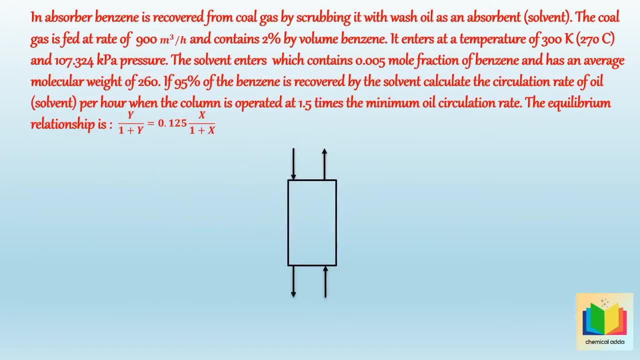 In absorber. Benzene is recovered from the column From coal gas By scrubbing it with wash oil is an absorbent That is solvent. The coal gas is fed at rate of 900 meters cube per hour And contains 2% by volume benzene. It enters at a temperature of 300 Kelvin. 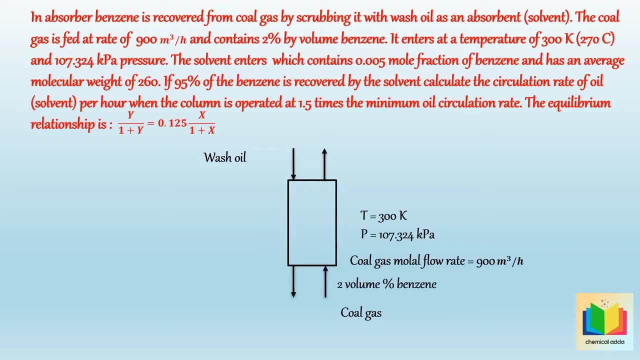 And 107.324 kilopascals pressure, The solvent enters, which contains 0.005 mole fraction of benzene And has an average molecular weight of 260.. If 95% percent of the benzene is recovered by the solvent, 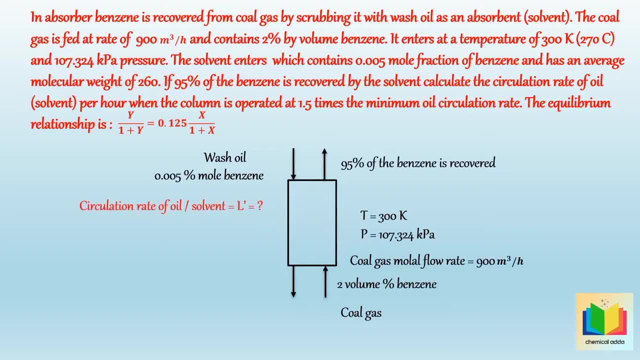 Calculate the circulation rate of oil that is solvent per hour When the column is operated at 1.5 times the minimum oil circulation rate. the equilibrium rate, 크, 파스�eted, Frontulam, lob, Visionاع. Africans Use minimum Master Control curve ratio, kops 만약. 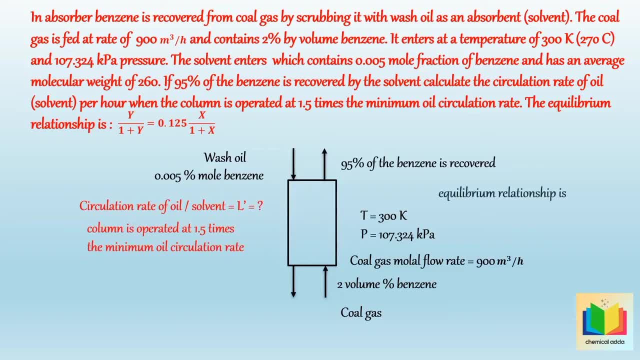 Now, if you want to measure the acid content around a column in a round terminal equilibrium relationship as given, where y is mole ratio of benzene to benzene free coal gas and x is mole ratio of benzene to benzene free solvent. hence, in this problem we have to calculate: 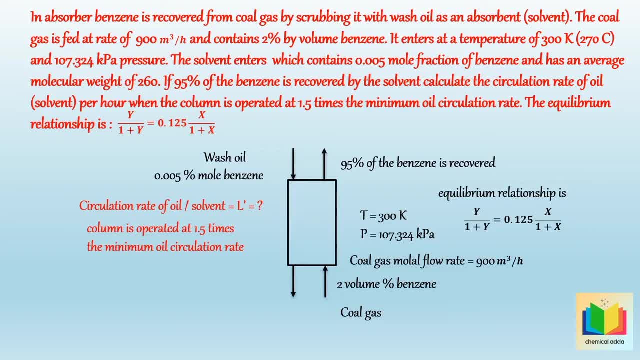 the solvent flow rate to the absorber when it is 1.5 times of the minimum oil circulation rate. that means first we have to calculate l minimum, then from this we can calculate l actual- that is actual solvent flow rate. now let's solve this sum. for that we take basis as: 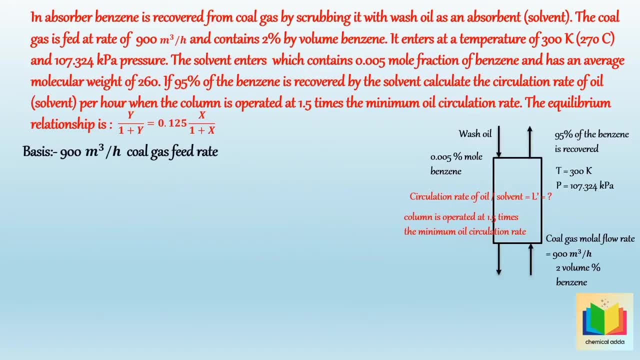 900 meters cube per hour coal gas feed rate. so to calculate l dash we take material balance of benzene over tower. v dash into y1 minus y2 is equal to l dash minimum into x1 minus x2. hence from this equation we can say that if we know y1, y2, x1, x2 and v dash, then we can calculate l dash minimum. 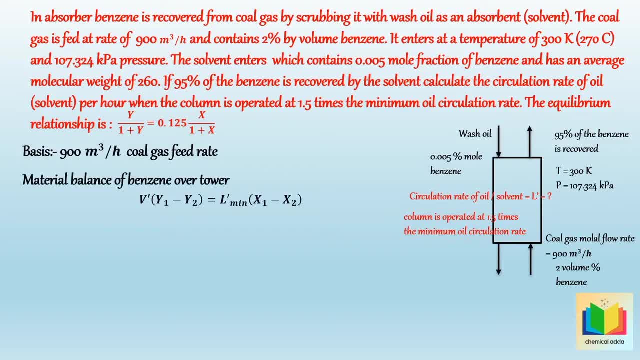 and from this actual solvent flow rate can be calculated. so let's find out these terms one by one. hence, let's first calculate y1. so, as we know, in this sum, given that inlet gas contain two percent by volume benzene, hence mole fraction of benzene in inlet gas, that is, y1 is equal to. 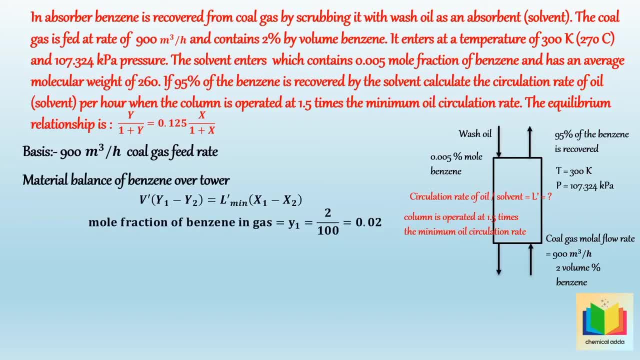 two, divided by l dash minus y2, x1 minus y2, x2 and v dash minimum, into x1 minus y2, x2 and v dash by 100, which is equal to 0.02. now from this we can calculate mole ratio, that is y1, which is equal. 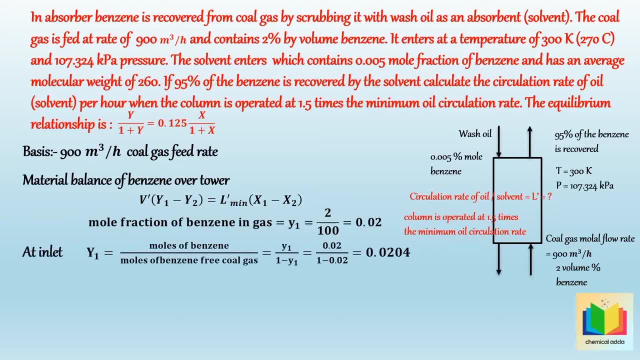 to moles of benzene. divided by moles of benzene free coal gas, which is equal to y1. divided by 1 minus y1, after solving, we get y1 is equal to zero point zero, two, zero four. now let's calculate y2, so as we have given ninety five percent of the benzene recovered. 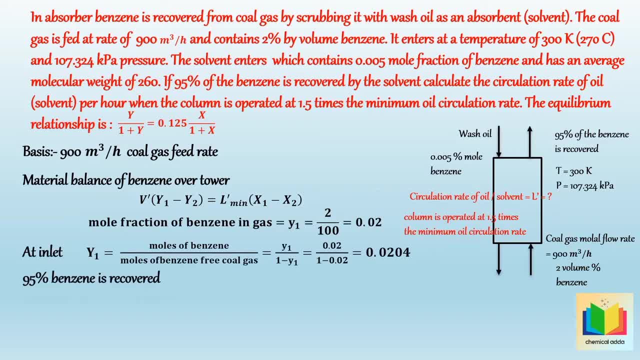 hence we can calculate: y2 is equal to one minus zero point nine five into y1. so after putting values and solving it, we get: y2 is equal to zero point zero, zero one, zero two. now let's calculate v dash, that is molar flow rate of benzene free coal gas. but in the sum we have given volumetric. 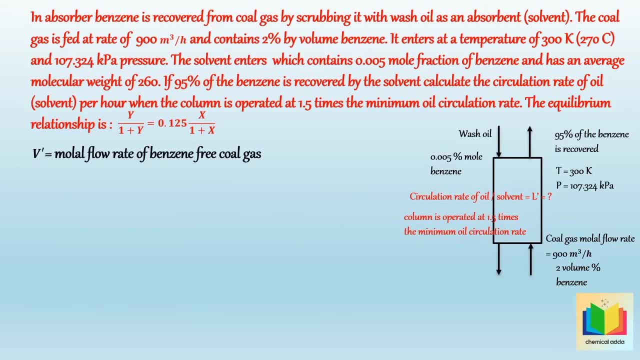 flow rate of coal gas, which is 900 meter cube hour. so first we have to find v, that is molar flow rate of gas. so from ideal gas equation we get: n is equal to PV divided by RT. so after putting values and solving it we get: n is equal to thirty eight point seven, two kilo. 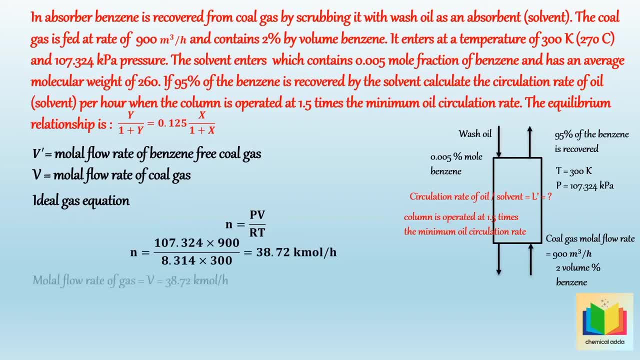 mole per hour. hence we get v, that is molar flow rate of gas, which is equal to thirty eight point seven, two kilo mole per hour. so we can calculate v dash, as v dash is equal to v, into one minus y1. so after putting values and solving it, we get: n is equal to thirty. 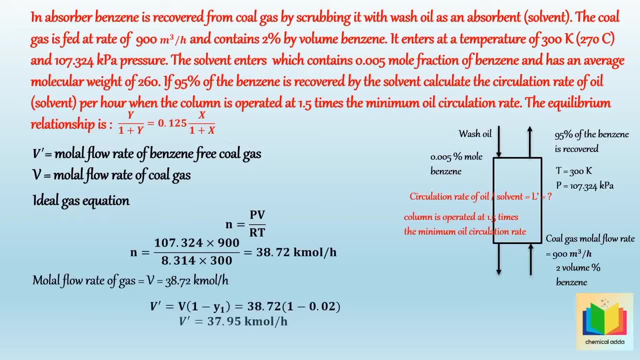 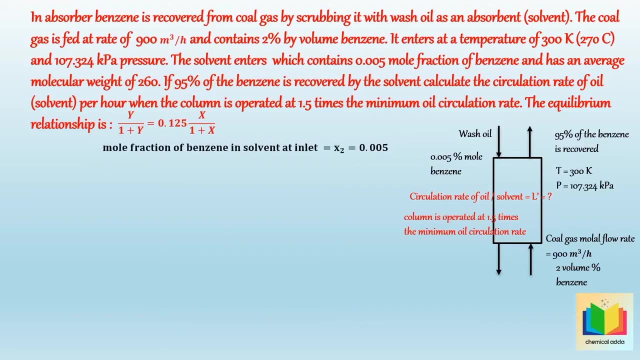 nine two, Steven mode by even heavy velocity, which is one van Shrimp ret headaches. we don't have order of mass and y2. in this case v dash is equal to cischer version. inspiresいう n, Kenneth Sohail. now let's calculate y2. so we have given mole fraction of benzene isolvent, we get v dash is equal to thirty seven point nine. 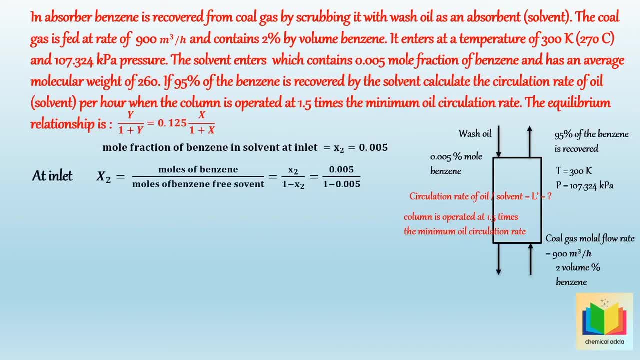 moles of benzene divided by moles of benzene free solvent. so after putting and solving it we get: x2 is equal to 0.005025. now let's calculate x1, that is mole ratio of benzene to benzene free solvent at outlet. so to calculate x1 we have to use equilibrium relationship. 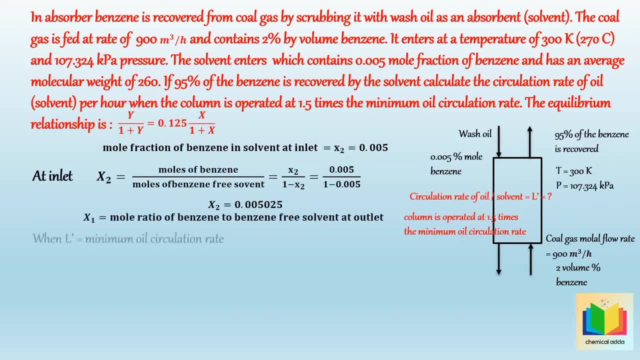 hence when i, that is, molal flow rate of benzene free wash oil is minimum from the equilibrium relationship we can write y 1 divided by 1 plus y 1 is equal to 0.125, into x 1 divided by 1 plus x2. 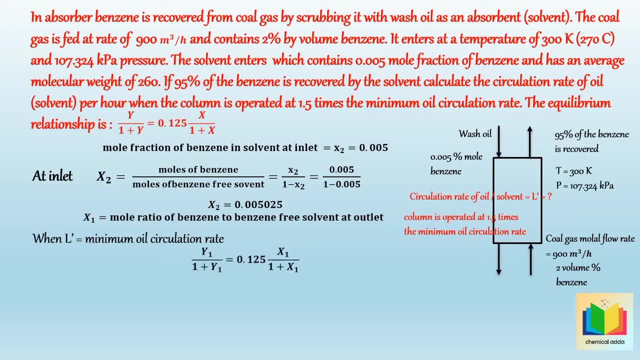 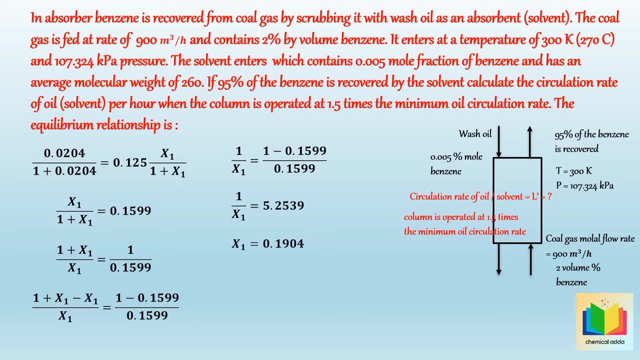 x1. so when y1 is equal to 0.0204, this relation can be written as so: after solving this equation, we get: x1 is equal to 0.1904. hence we get all values, that is, x1 is equal to 0.1904, x2 is equal to 0.005025, y1 is equal to 0.0102, v dash is equal to 37.95. 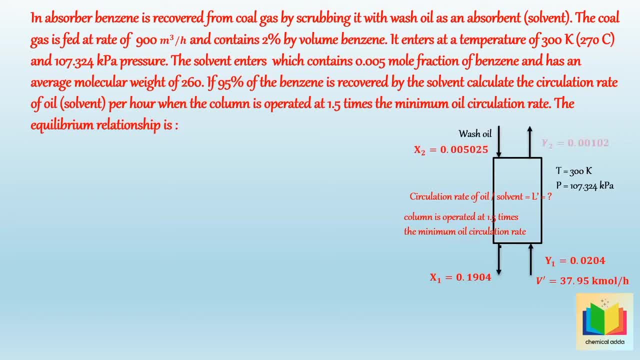 kilomole per hour, y2 is equal to 0.0204. hence now we can calculate: l dash minus x1 is equal to 0.0105, x2 is equal to 0.0105, x2 is equal to 0.0105, x2 is equal to. 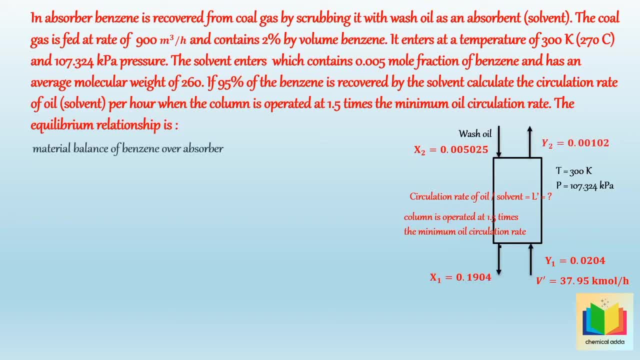 minimum. so from material balance of benzene over absorber we get. after putting values and solving it, we get l dash minimum was equal to 3.97 kilomole per hour. hence we get minimum flow rate of benzene free solvent, that is, l dash minimum was equal to 3.97 kilomole per hour. now from 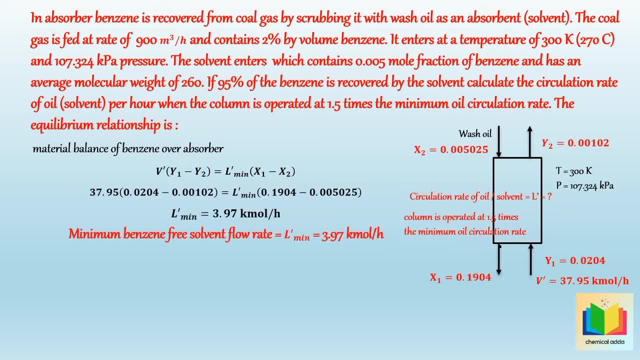 this. let's calculate actual flow rate of benzene free solvent. that is l dash actual. so we have given the column is operated at 1.5 times the minimum oil circulation rate. hence we get: l dash actual is equal to 1.5 times l dash minimum. so after putting values and solving it, we get: 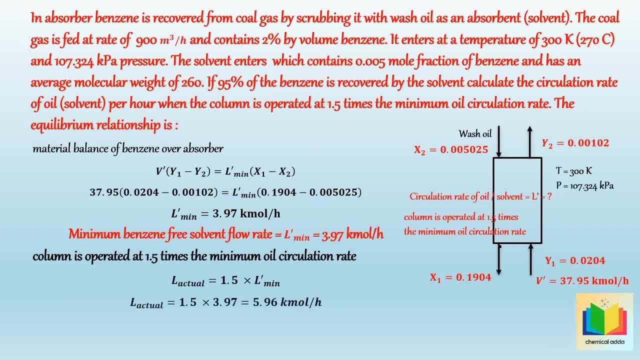 l dash actual is equal to 5.96 kilomole per hour. hence we get actual flow rate of benzene free solvent will to 5.97 kilomole per hour. if we multiply it by average molecular weight, that is 260, we get actual flow rate of benzene free solvent is equal to one thousand three hundred.